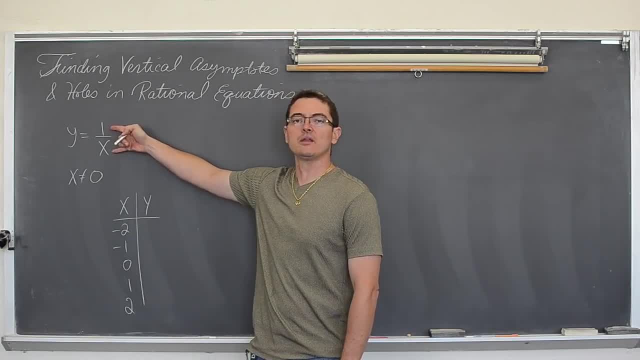 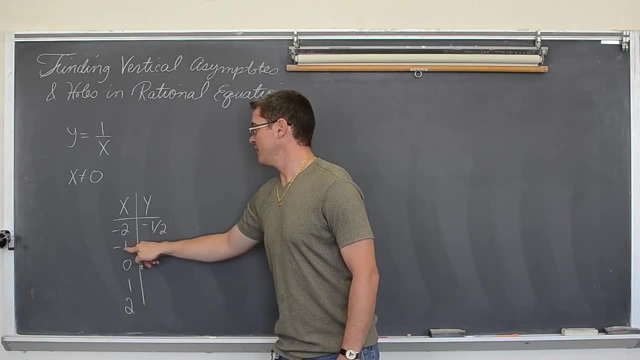 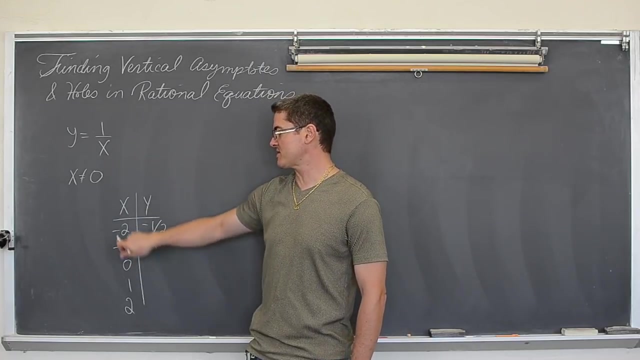 And let's just plug those in. If you plug in negative two, you get a y value of negative one half. If you plug in negative one, one divided by negative one is negative one And I included zero. but we already know that that is undefined. 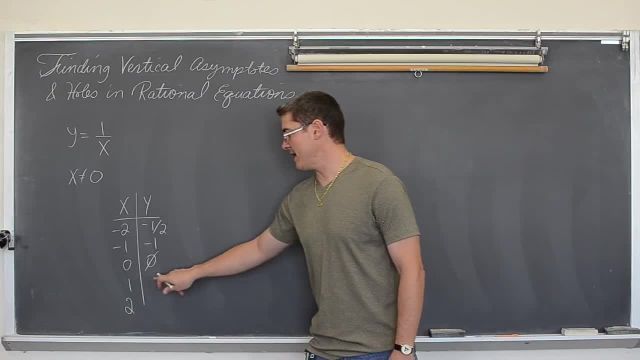 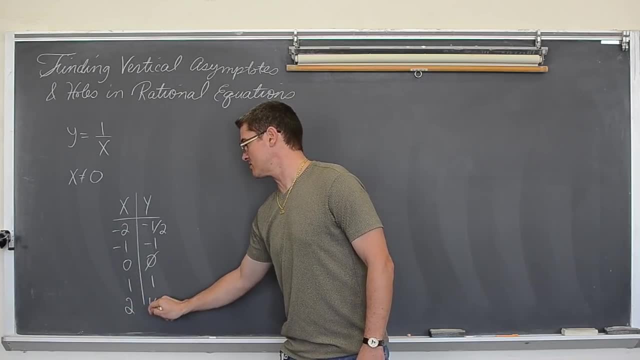 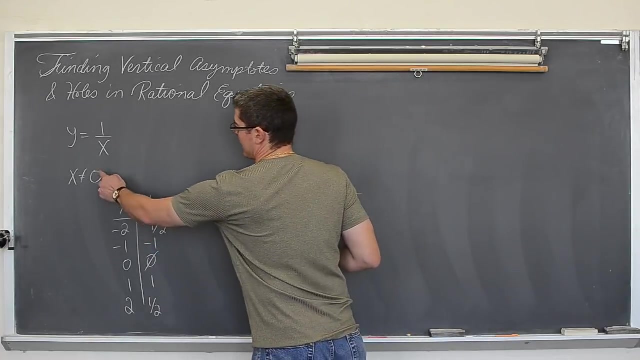 So that just simply doesn't work. And we have the values of one: One divided by one is one, And one divided by two is one half. Let's see if that is enough to get an idea of what is going on here. Well, I can't have x equal to zero. I cannot divide by zero. 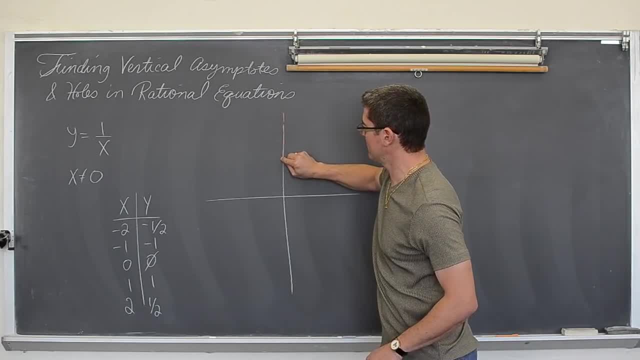 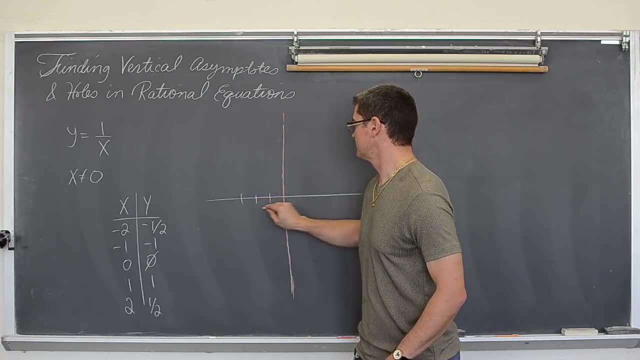 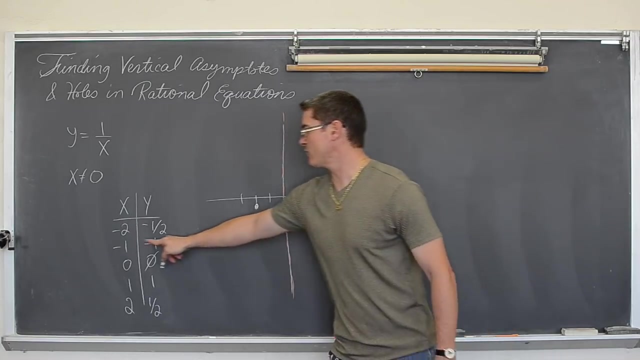 So this graph will have a vertical asymptote at x equals zero. But then what happens after that? Well, at negative two, we are at negative one half, We are at negative one half, And at negative one, we are at negative one. 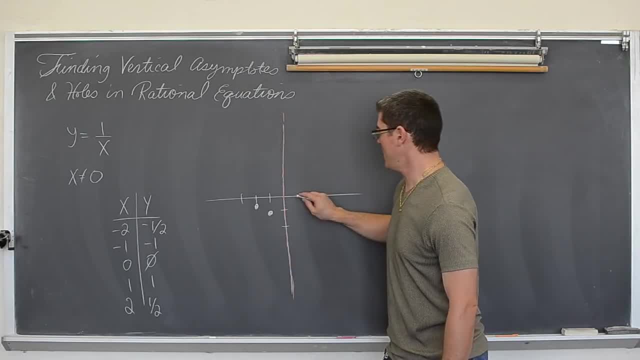 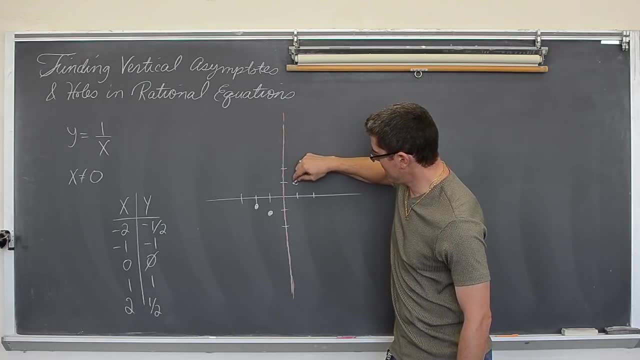 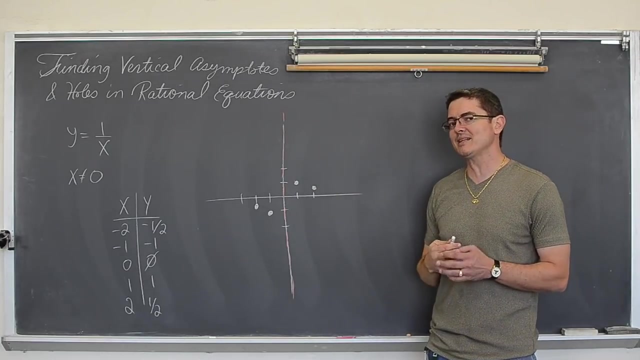 At zero, we are undefined. And at positive one, we are at one, And at positive two, we are at one half. So one one and two, one half. Is that enough to actually let you see what is going on? Well, probably not. 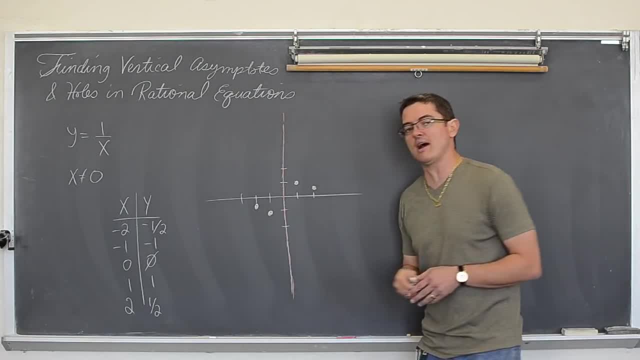 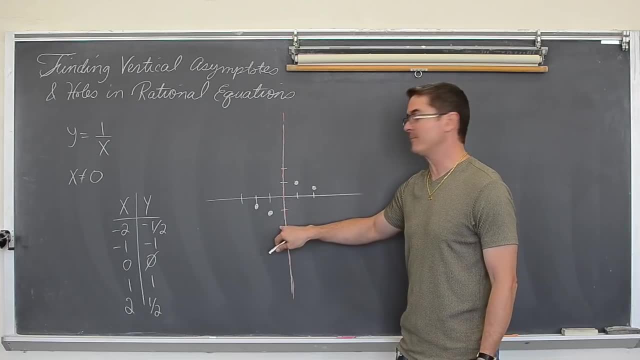 Because you may never have seen vertical asymptotes in your graphs before, So we might need a couple more points. So let's add a few more. What happens as you get closer to zero from the left and the right, Like what happens if x is equal to negative one half? 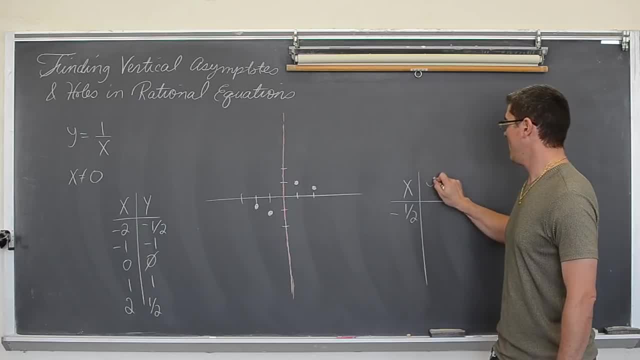 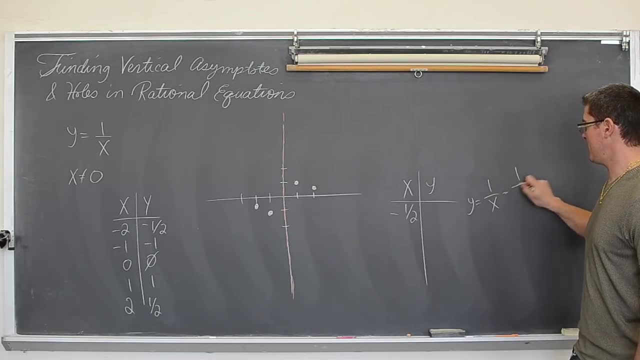 So, as we creep a little bit closer to the vertical asymptote, Well, that is going to be: y is equal to one over x, That is going to be one over negative one half. And I have explained before, like how it is top divided by bottom. 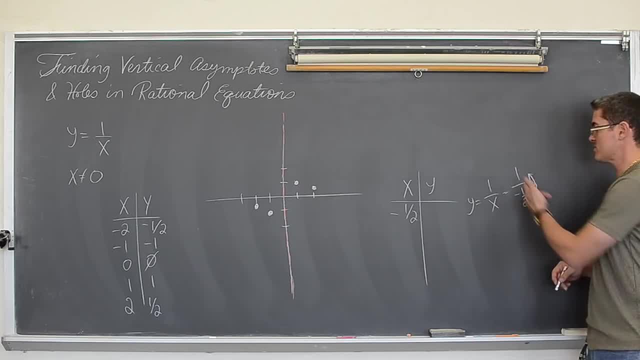 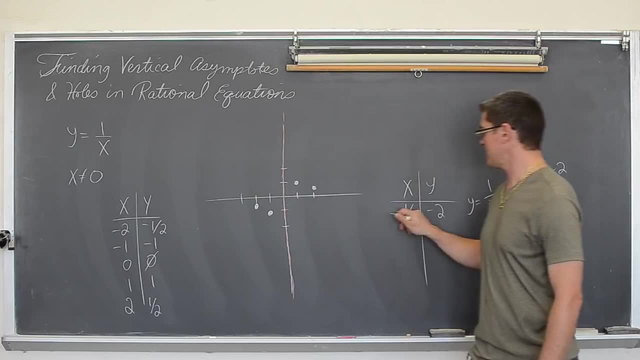 You can't really divide fractions. That is going to flip up the bottom. So one divided by one half is the same as negative two. Okay, so as I get closer, where x is negative one half, my y value is getting to be negative two. 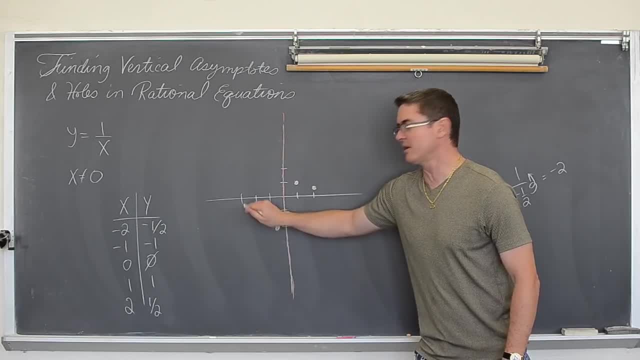 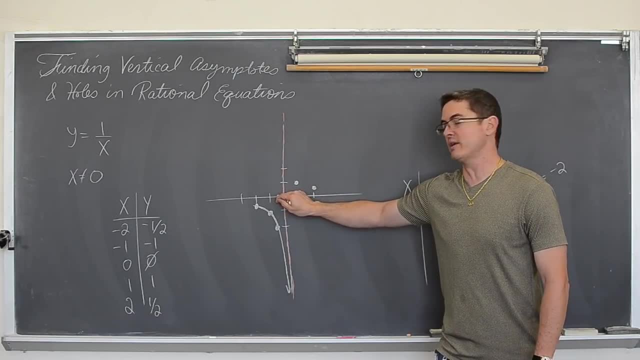 And now, if I connect these points, you can see that there is a little bit of curvature happening. That graph is going to. If you can put in negative point five, Or negative one half, negative one fourth, negative one tenth, You are going to see that your values become more and more negative. 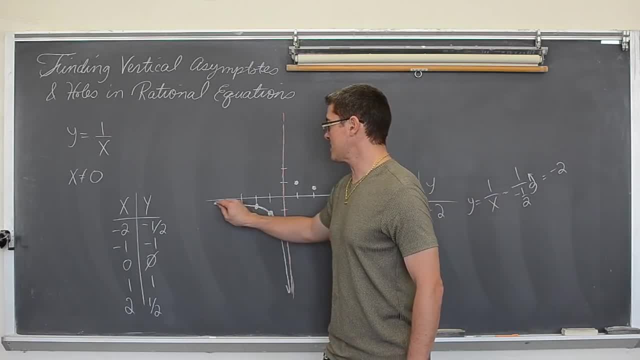 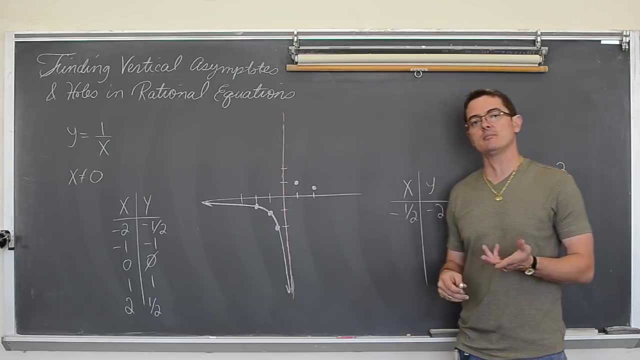 And actually go down to negative infinity. We will be talking about horizontal asymptotes, but not in this video. So I know that this graph is going to flatten out and approach the x axis from the bottom, But we haven't talked about vertical asymptotes yet or horizontal asymptotes. 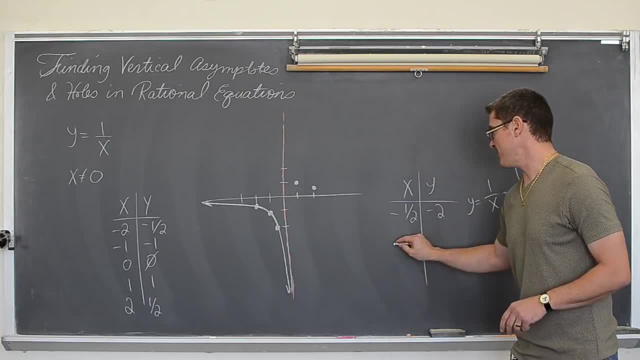 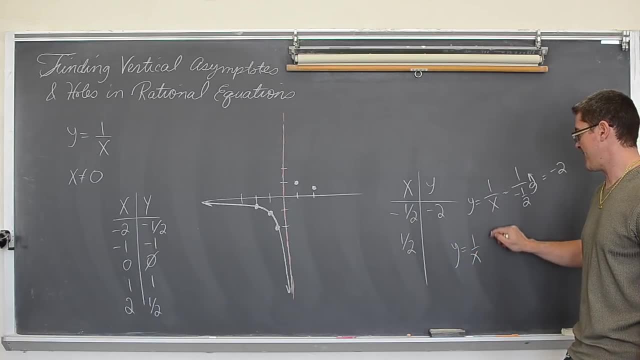 So for now, I am just going to take my word for it. What happens at positive one half? Well, again, x is equal to one over x, And that is now going to be one over one over two. x value one half. 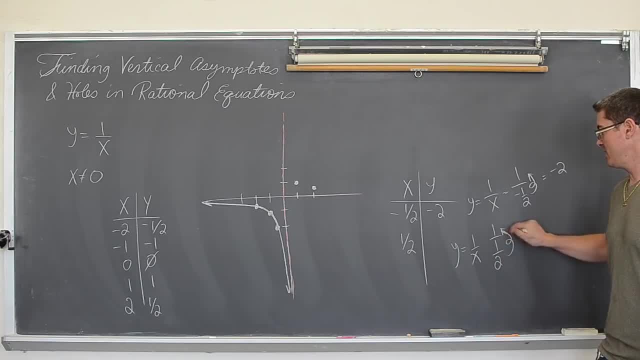 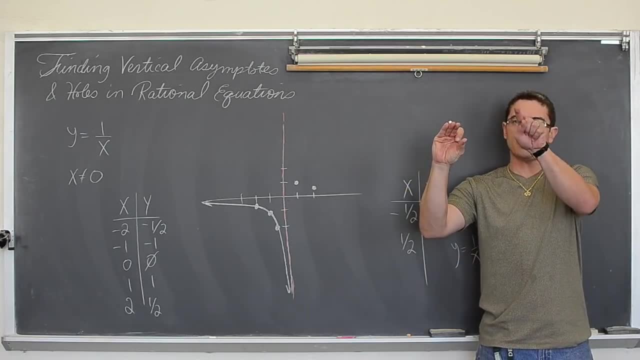 And when you have a fraction or just a number over another fraction, you want to flip that bottom fraction up, Because you can't really divide by fractions. Well, one divided by one half means you would have to change that division to multiplication and flip that second number. 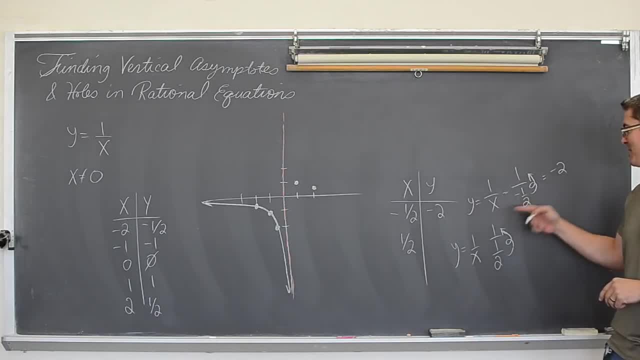 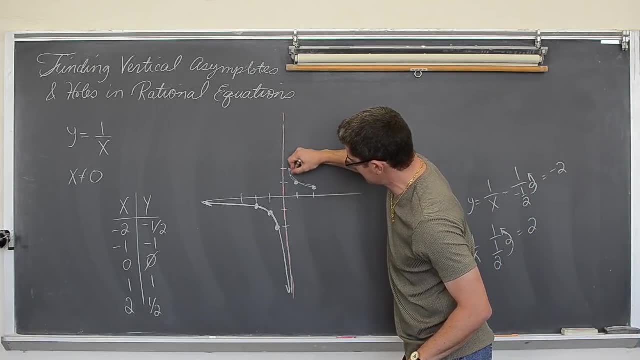 If you remember fractions from many, many years ago. So you flip the bottom up and you get two. So at one half we are at two And again you can see this curvature happening And we are going to hit the Well. actually, we are never going to hit the vertical asymptote. 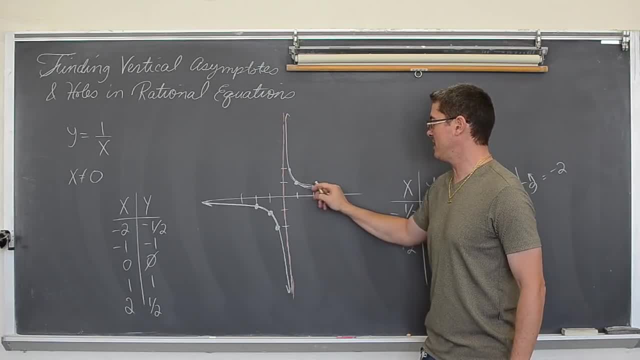 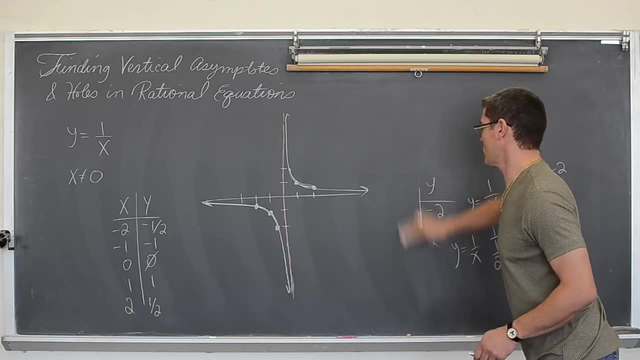 But on the right hand side we are shooting up to positive infinity And then that line is going down to the right. You can also double check that with a graphing calculator, if you have one. Of course we are not doing all this work for graphing rational functions. 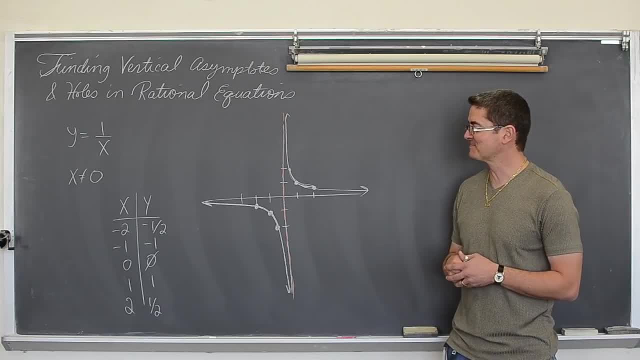 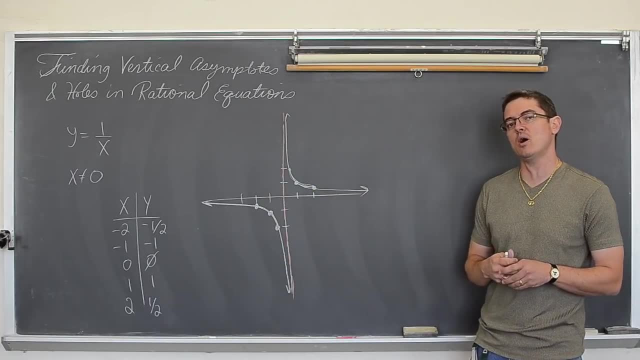 If we can. just You know the calculators will be our check. Ok, So we have y equals one over x And a table of values trying to show you that the vertical asymptotes show up where the denominator is equal to zero, Usually. 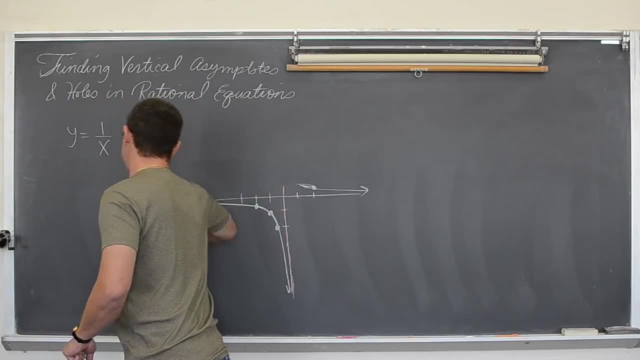 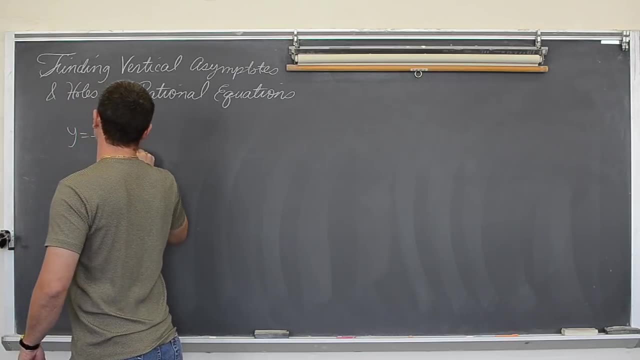 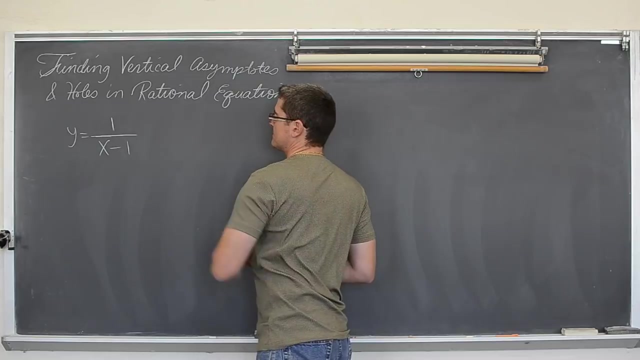 What about if it were: y equals x minus one, Where I am taking the function and within the function I am adding a negative one? It is just a simple negative one. Well, If you remember what I just had up here a second ago, 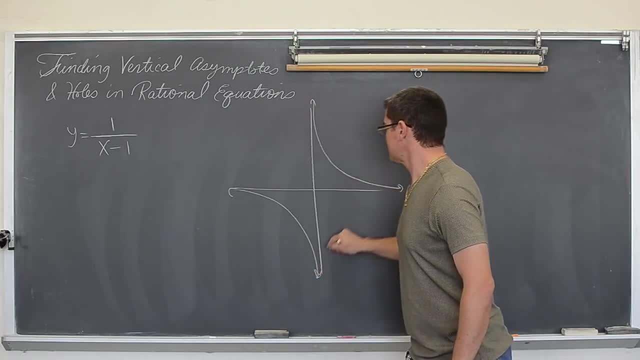 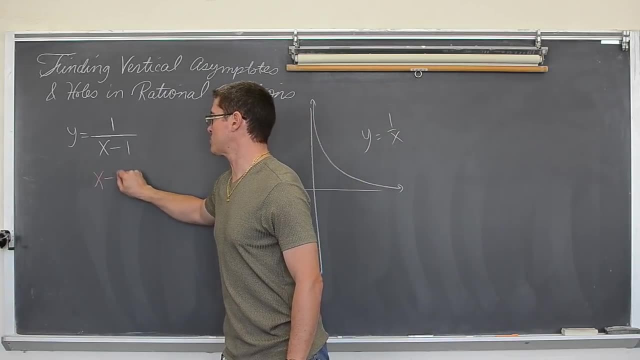 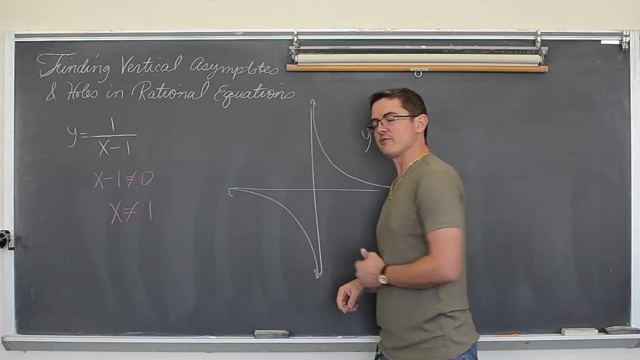 This is: y equals one over x. Well, again, you cannot divide by zero, So x minus one cannot be zero, So x cannot be one. So now, instead of before, where the vertical asymptote was at zero, Now my vertical asymptote is going to be at x equals one. 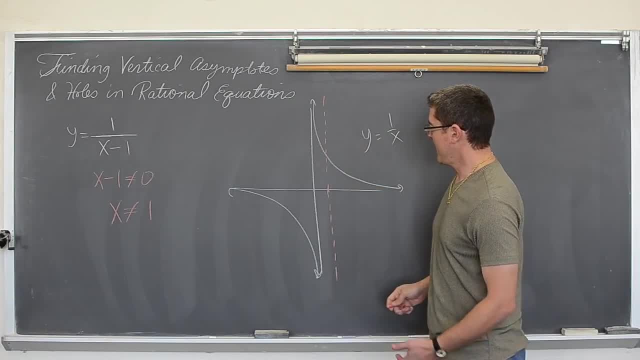 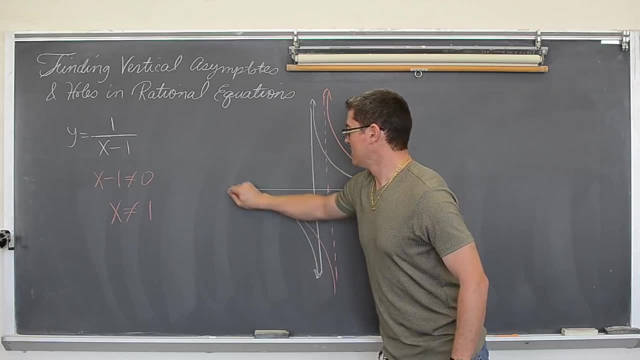 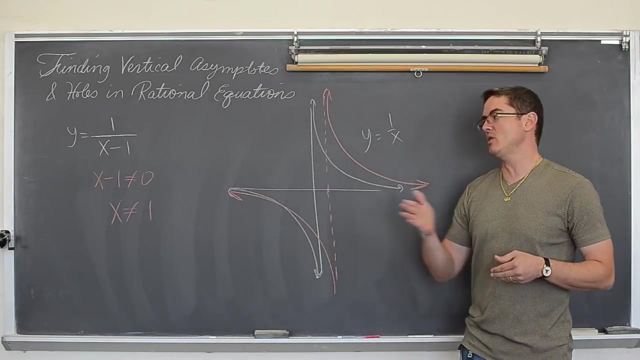 And the graph is going to just simply move to the right Now. if you remember your sections about transformations, You will know that if you have a plus or minus inside the math function, that is a movement left and right. So when you see a negative one inside this basic function, 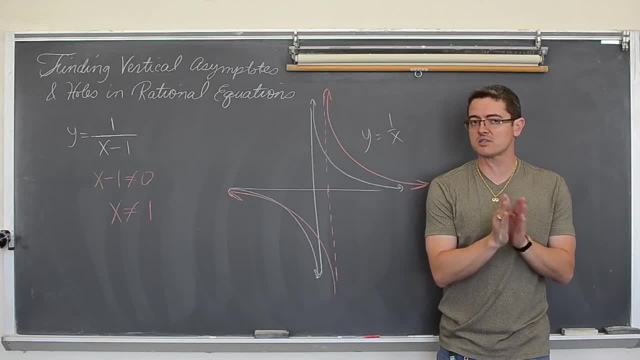 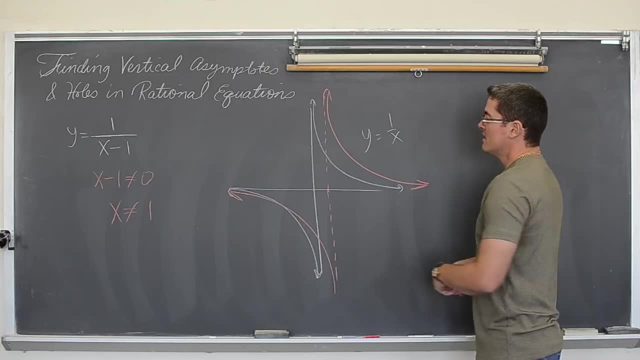 It was one over x and now it is one over x minus one, Just that subtraction inside the function. You should have expected that that horizontal shift of one to the right. So again, denominator equals zero. I did not do a t table with this one, because it was just a shift. 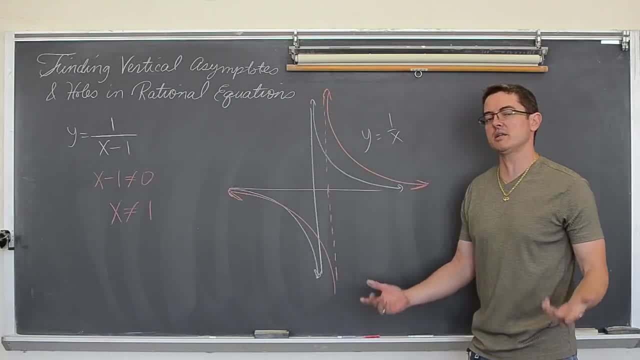 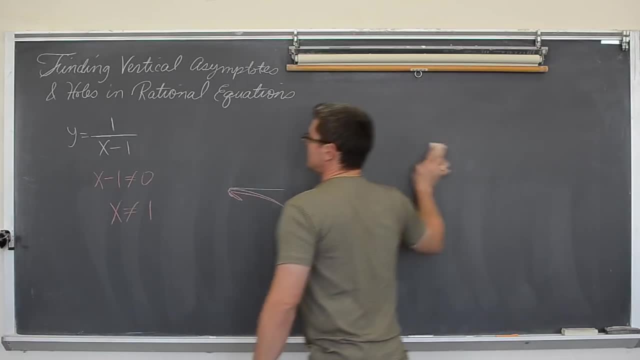 And our vertical asymptote now is at x equals one instead of x equals zero. Ok, So one more example like that. This time I am going to cheat and use my graphing calculator to give me a table, But we are going to have 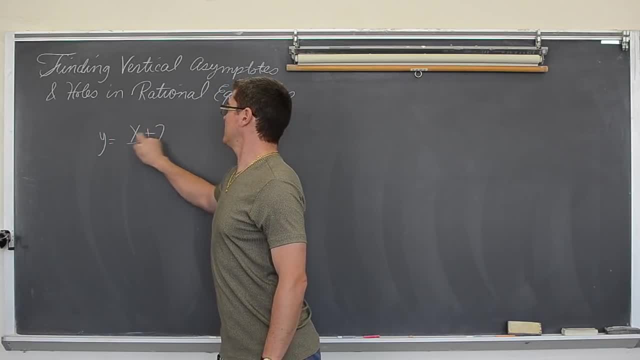 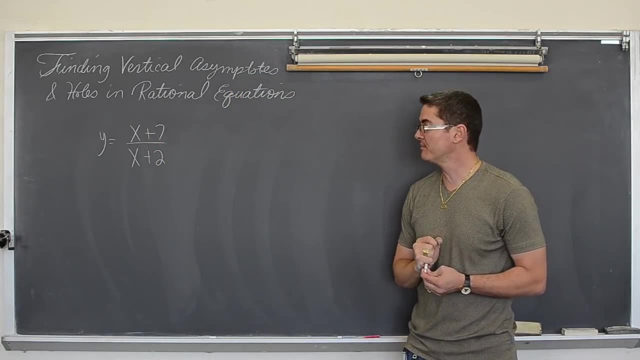 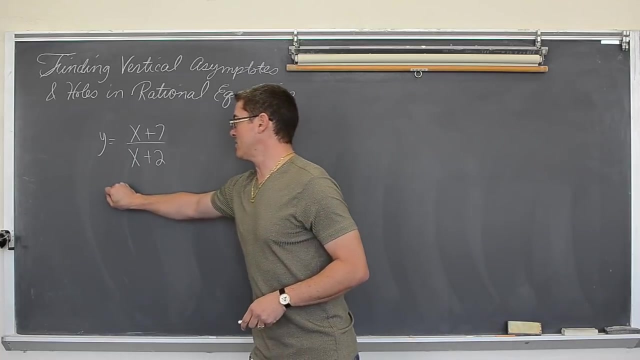 Y equals x plus seven over x plus two. Now again, I told you cannot divide by zero. Now, if I can make this body equal to zero, Then that is probably a vertical asymptote. So x cannot, or x plus two cannot, equal zero. 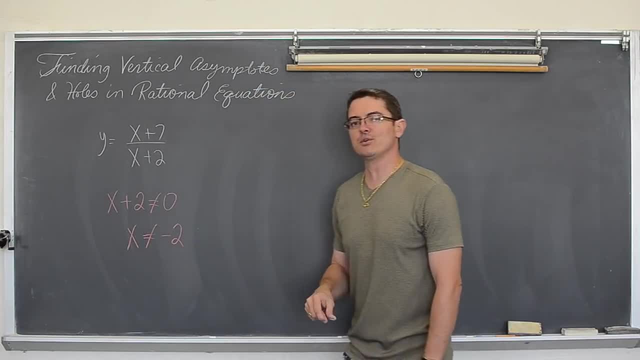 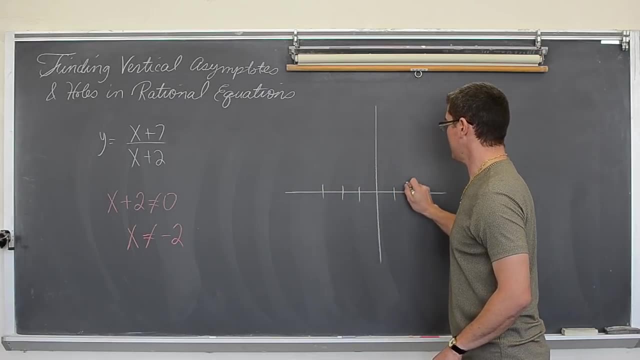 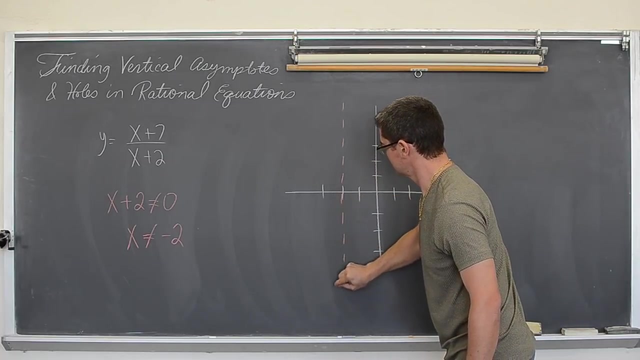 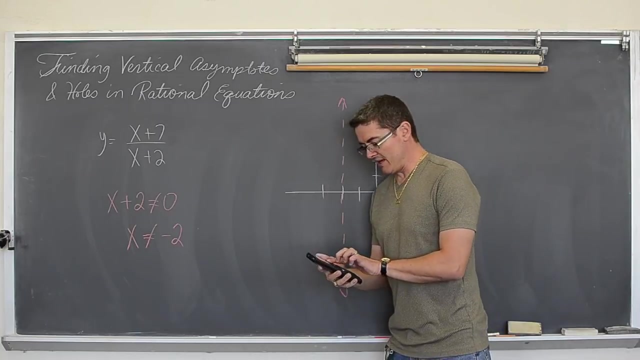 So x cannot equal negative two And I contend that at negative two There is going to be a vertical asymptote Because I cannot divide by negative two. So if I use my handy dandy calculator here And go to my current diagrams, 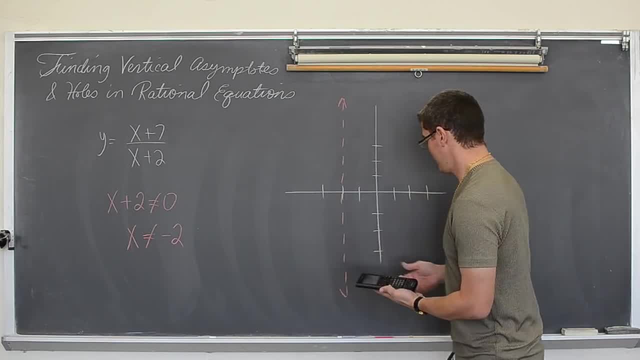 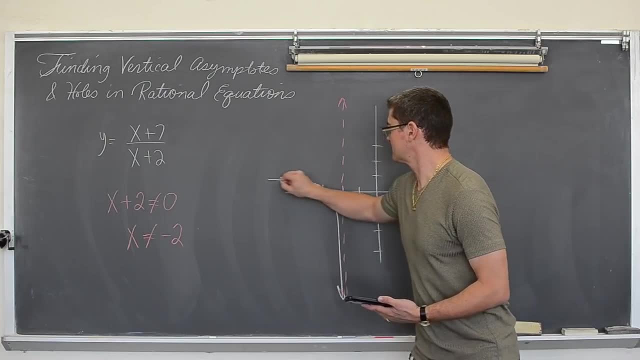 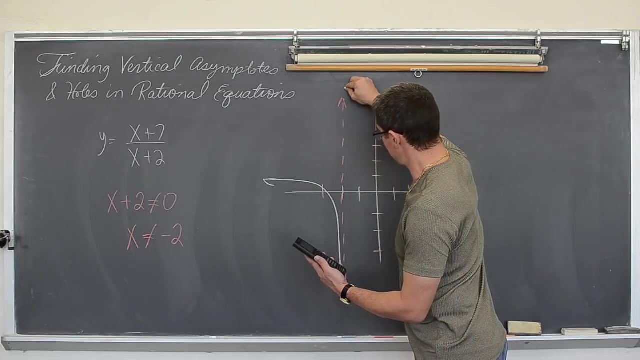 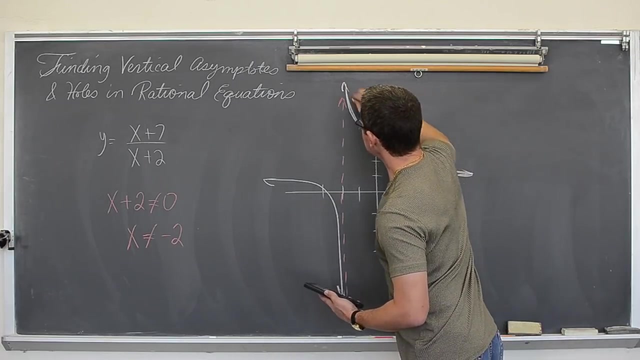 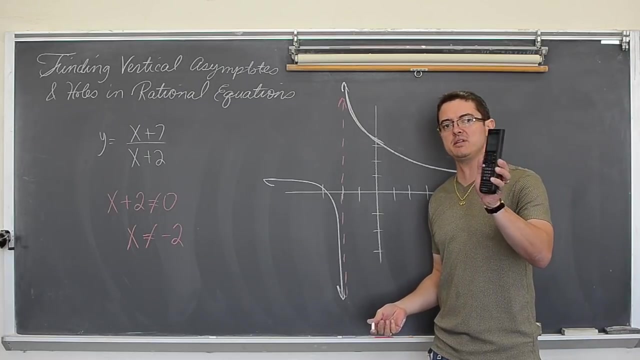 Why? yes, This graph is going to Approach and go down Against the left side of the asymptote And come up and look something like this, Approaching And shooting up towards the right hand side of the vertical asymptote, You might be going: hey, you are not really supposed to be using t tables. 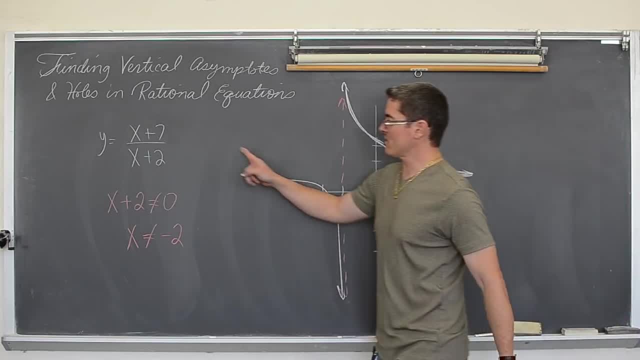 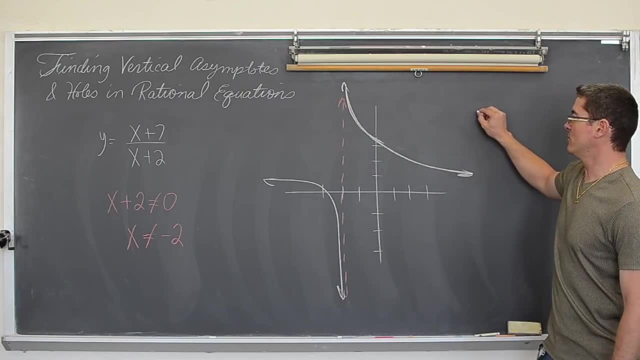 Well, no. So what you might do is: Ok, I know there is a vertical asymptote at x equals negative two. So for a sketch of the graph, You can do some. Make up some x values Such as: ok, the vertical asymptote is at negative two. 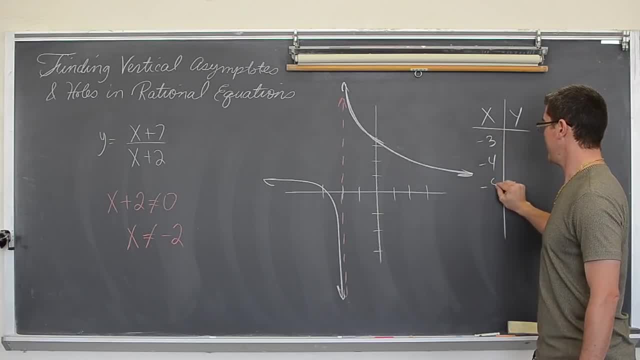 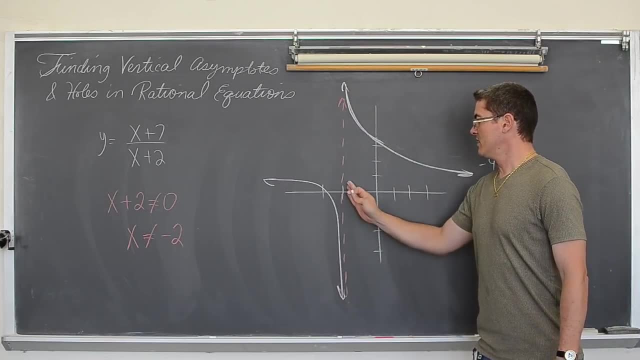 So try: negative three. Negative four. Negative five. Now I would like to put these in order, So it is kind of annoying. I just wrote it like that: On the right hand side of the asymptote, To the right of negative two. 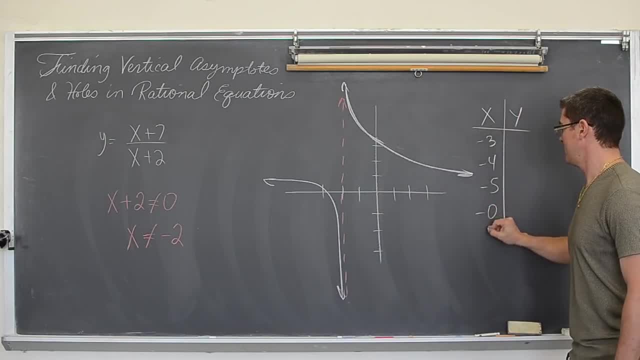 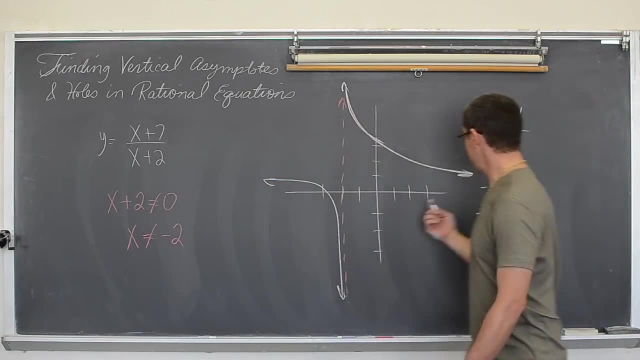 Maybe you can try some values of negative one, Zero and one And then plug each of those in one at a time into the equation. Like negative one Would be negative one plus seven Over negative one plus two. So that is six over one. 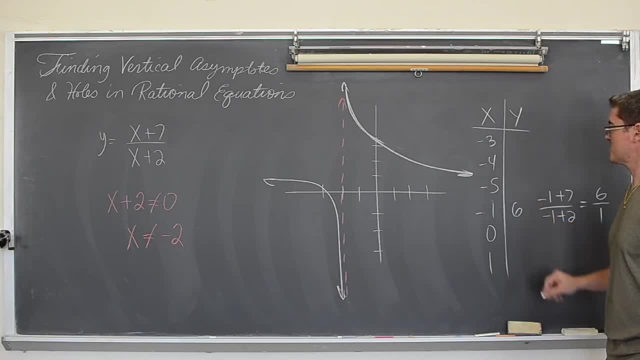 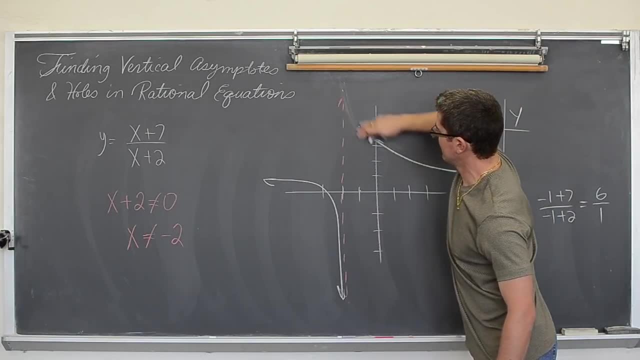 So at negative one. We are at six, So at negative one. My drawing is certainly not drawn to scale very well, Would be up here at, So let's just fix it. Negative one: One, two, three, four, five, six. 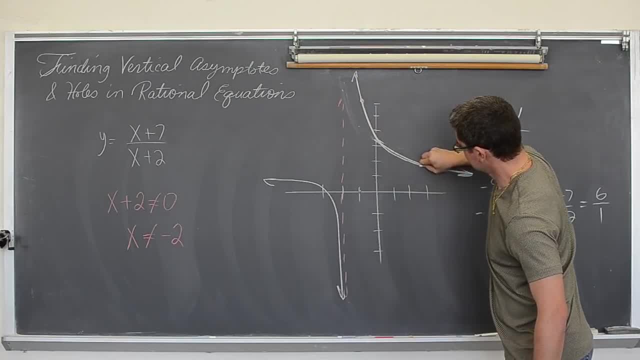 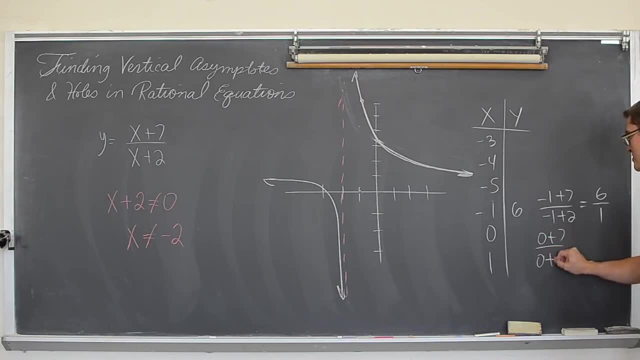 So the graph actually looks like this, And then I can plug in zero And work it out: Zero plus seven over zero plus two, Which is three point five, And so on. So I am using some values to the left of the vertical asymptote. 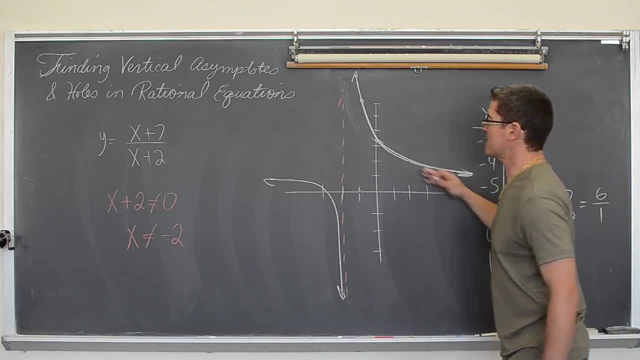 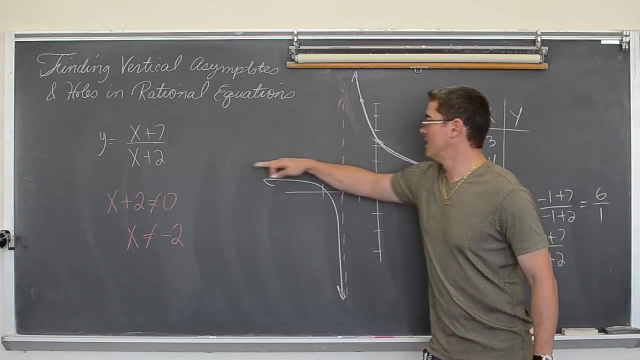 And I am using some values to the right of the vertical asymptote To kind of get an idea of what the graph is doing. For a complete idea You have to know what is going on here And why is this curving and flattening out of the graph happening at this value? 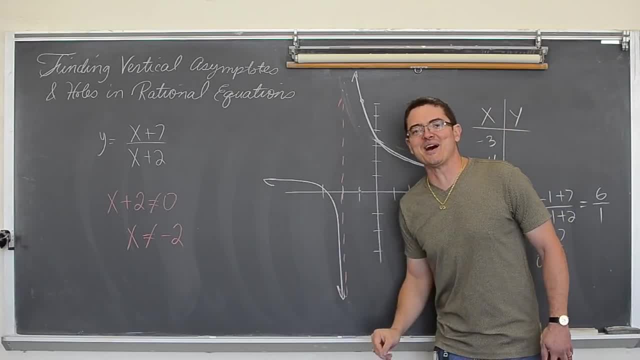 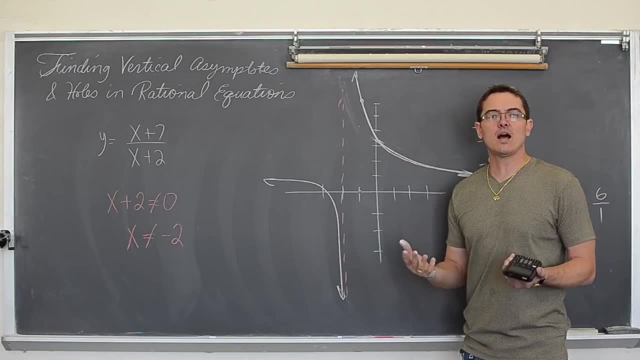 What appears to be y equals one. Well, I will take care of that when I cover horizontal asymptotes in another video. Ultimately, we are going to do a few parts And then do like one video where I graph one or two rational equations from start to finish. 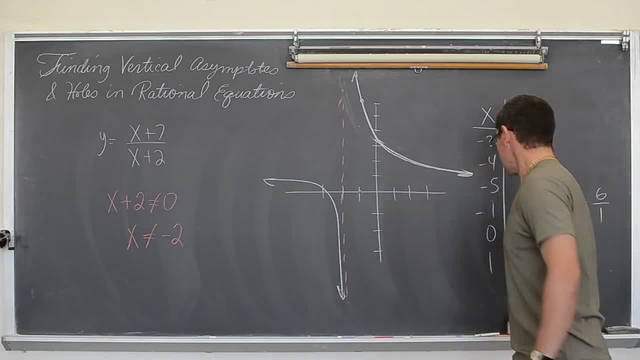 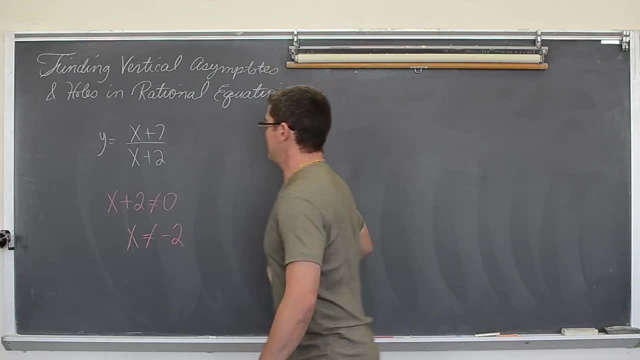 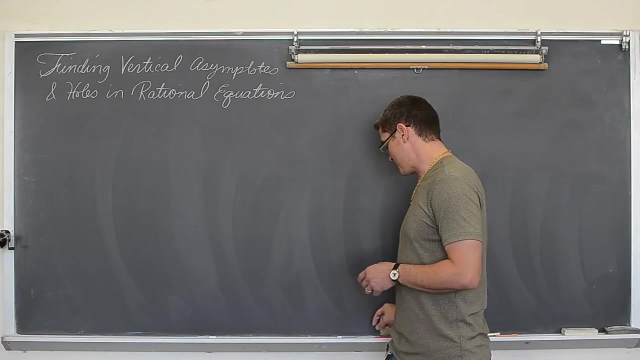 That video is probably shot on Friday. So that is three examples of how, when you have A vertical asymptote- Or, excuse me, The denominator equals zero- You have a vertical asymptote. Well, how about an example where we don't get a vertical asymptote? 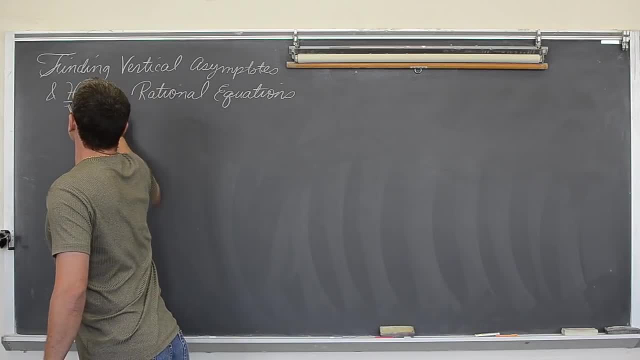 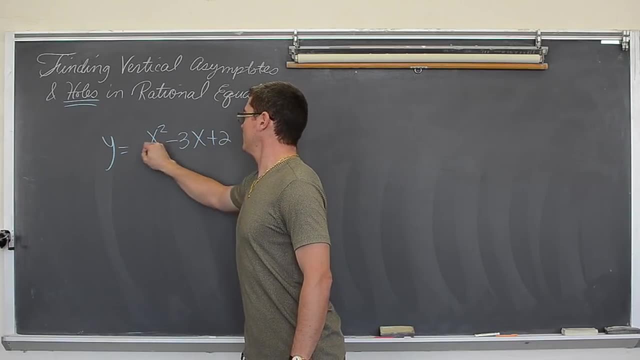 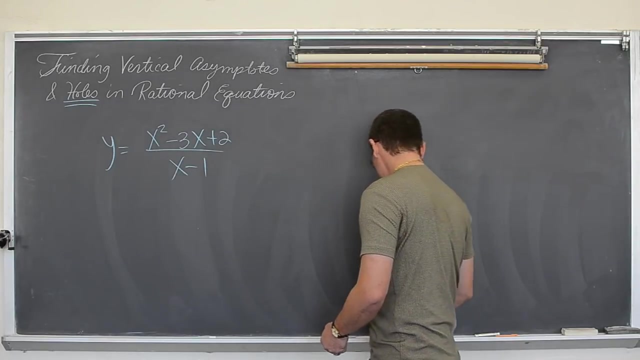 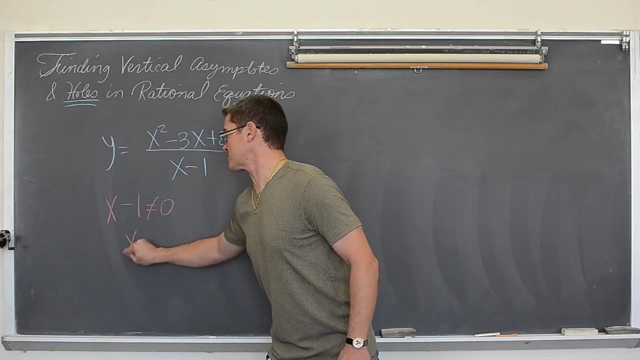 We get a whole. So y equals x squared minus three, x plus two over x minus one. Well, I can make that denominator equal to zero. I cannot use X minus one cannot equal zero. So x cannot equal one. So something is going to happen at x equals one. 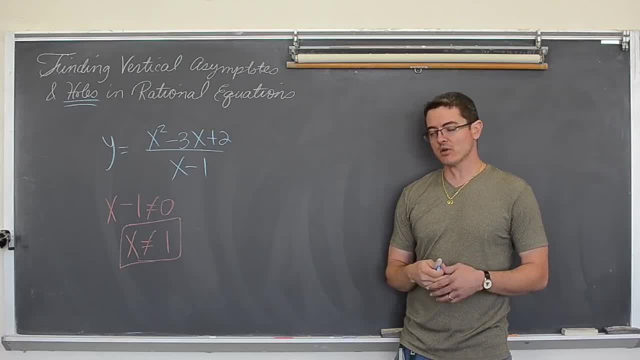 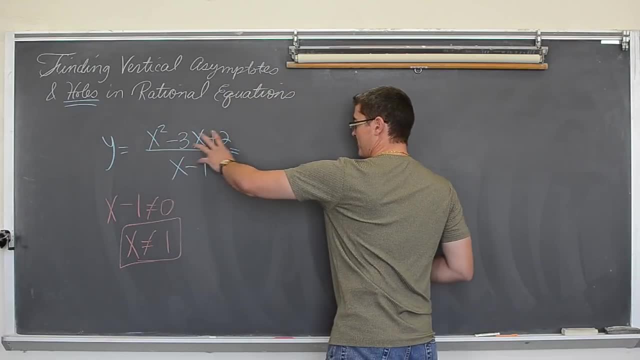 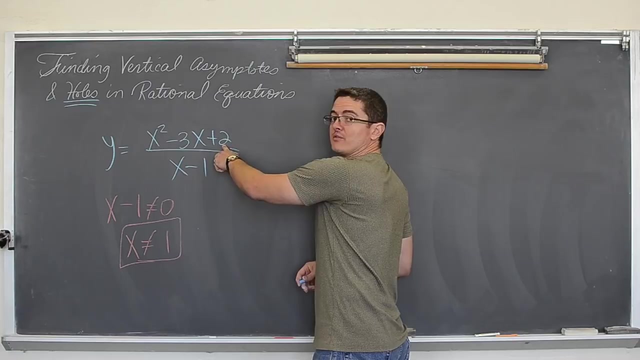 Is it going to be a vertical asymptote again? Well, in this case the answer is no, And the reason why is going to be found through the simplification process of this rational equation. This top trinomial factors. There are factors of two. 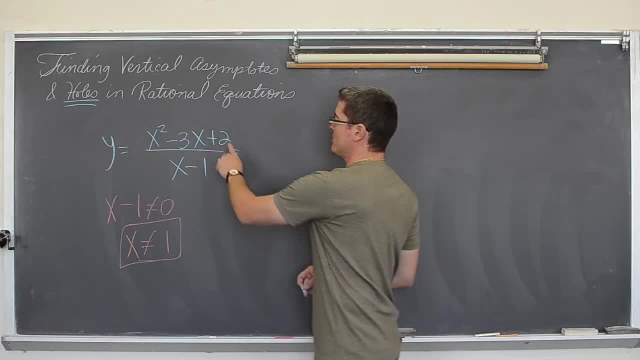 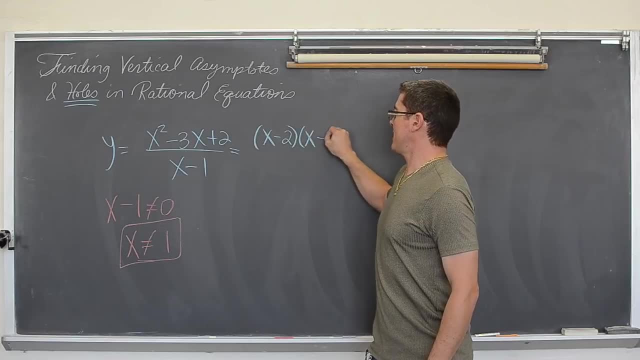 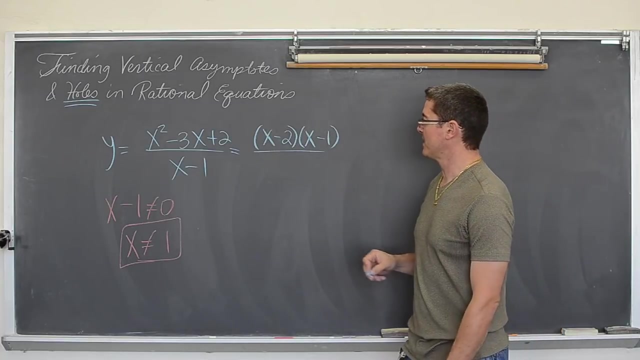 That add to negative three, And I can do that simply because the leading coefficient is one. The top will factor to be x minus two times x minus one, And you can double check that. That will multiply back together to give you x squared minus three, x plus two. 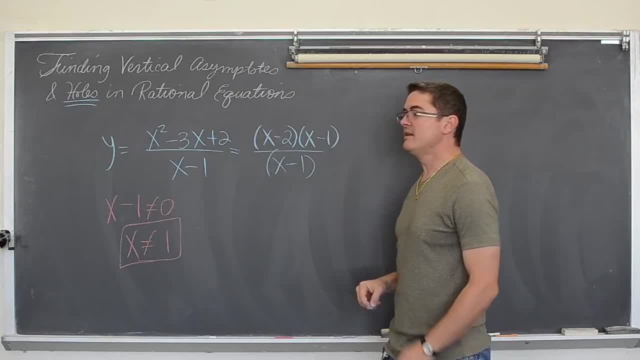 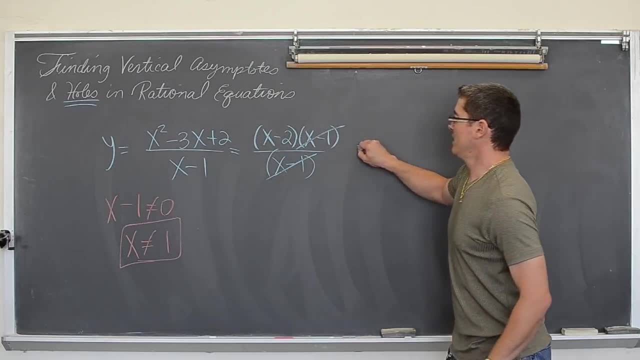 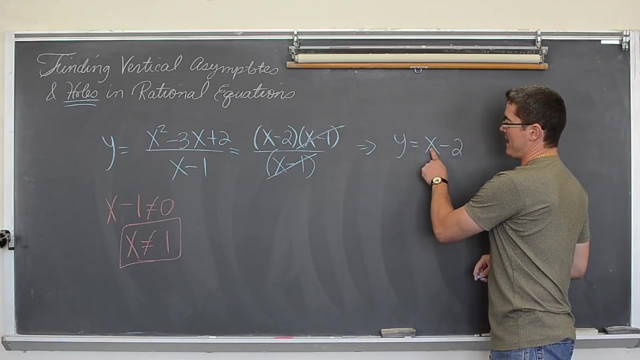 That is over x minus one. And now see my x minus one is factoring out. My simplified version of this equation Is: y equals x minus two. Well, that is, y equals mx plus b. This is slope intercept form. This is simply the equation of a straight line. 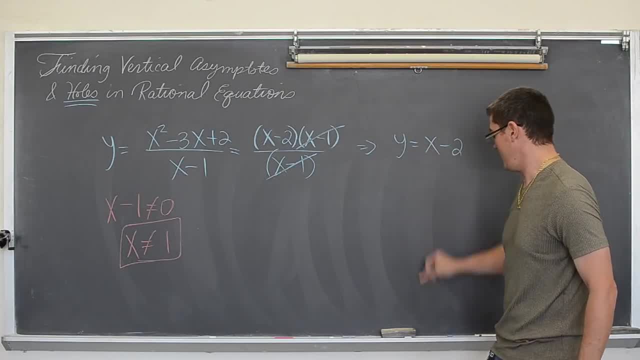 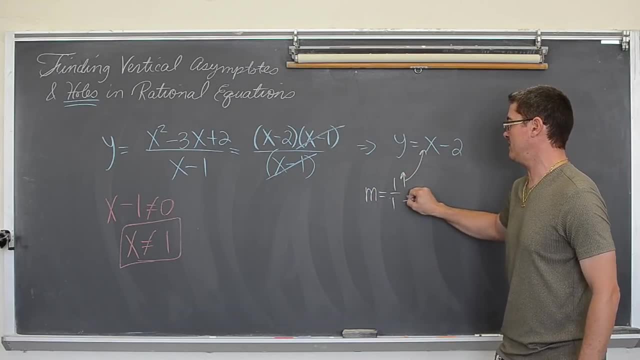 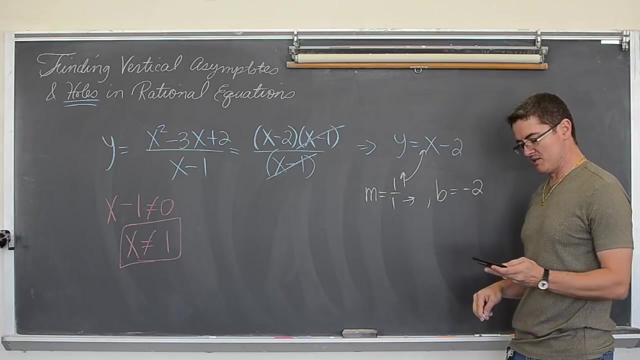 So I can graph this by going: hey, the slope is equal to one over one, So that is going to be up one and over one. The y intercept, or b, is equal to negative two And that means that this is going to. The video is going to be done in a second.